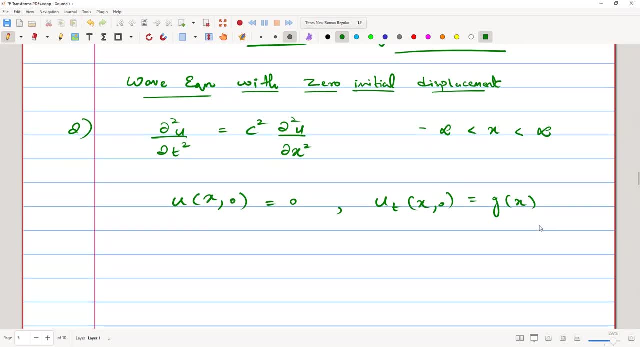 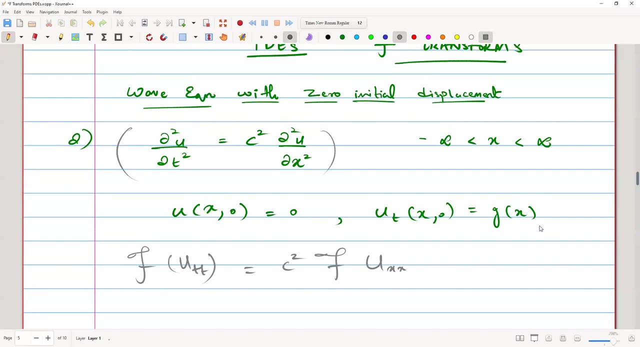 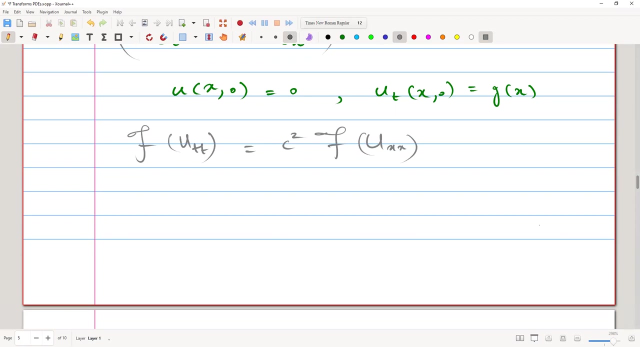 g of x right Now, doing the same thing. first, we will apply the transformation on the equation and we know when we apply transformation on this equation, we will simply get a second order, ordinary differential equation with constant coefficients and obviously it will be homogeneous equation. So the transform of this derivative is: 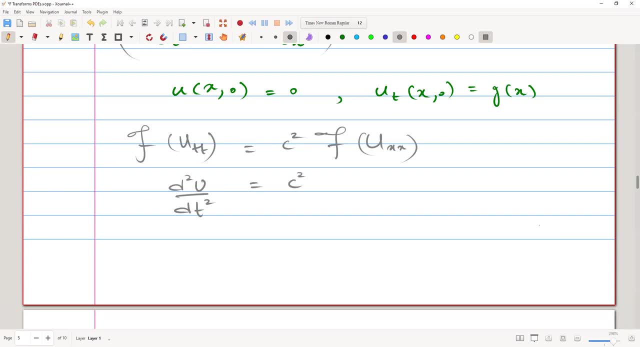 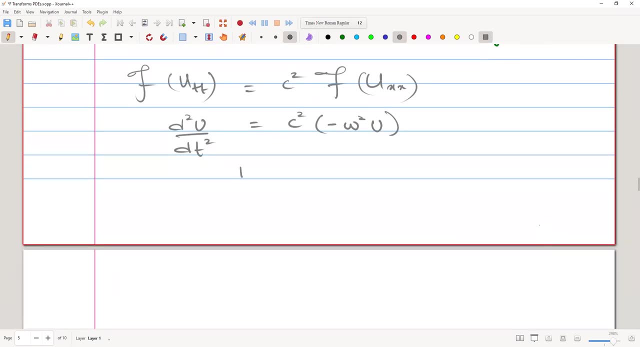 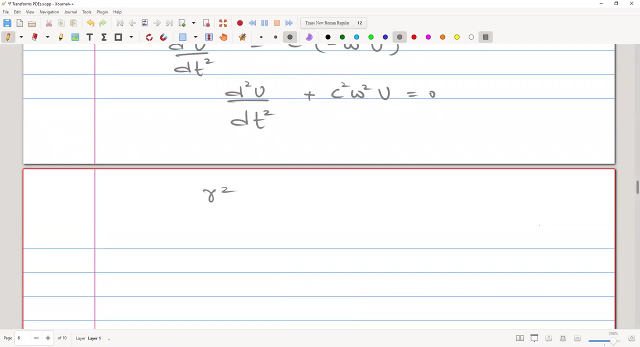 d squared u over d, t squared. and here we have negative, omega squared u. So now the differential equation. we can see it is second order and with constant coefficients and homogeneous. So we can easily solve this equation by making auxiliary equations. So it will be negative, c squared, omega squared. So the roots of the equation. 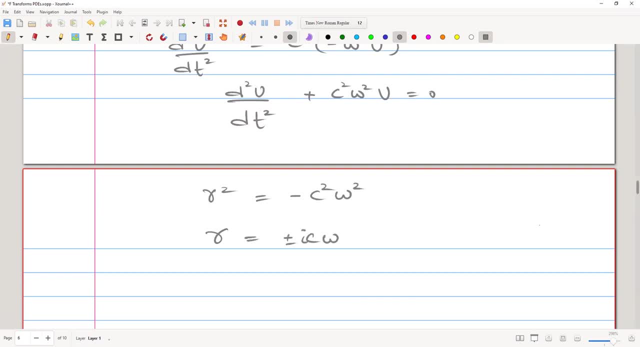 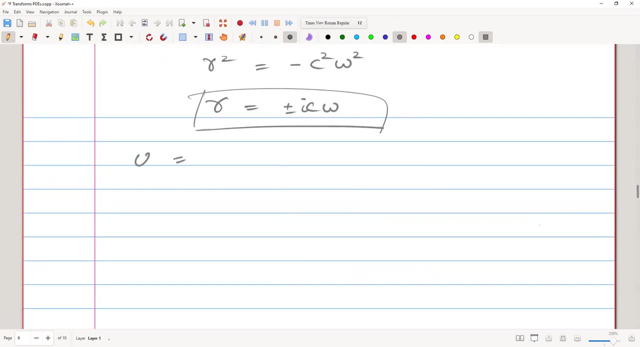 will be plus minus c omega, with iota here Right, so complex because of this negative sign, and we can write the solution as a cosine omega c t plus b sine omega c t. And now what we need to do is we need to apply the Fourier, apply the initial conditions, but before doing that, we need to apply Fourier. 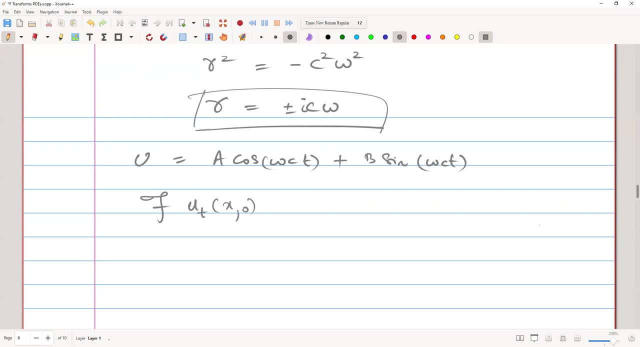 transformations on the given initial conditions. so we need to apply the transform on the initial velocity. that is a function of X. so apply the transformation. we will get G of Omega here, like this right. and if we apply the transformation, or for ux, comma zero, that is initial displacement. 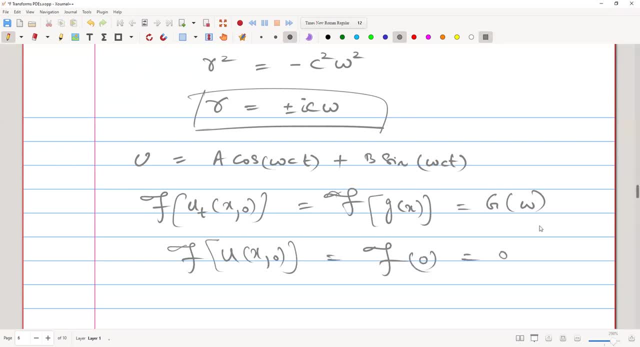 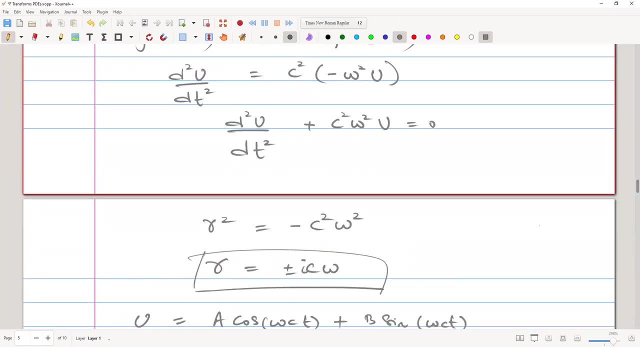 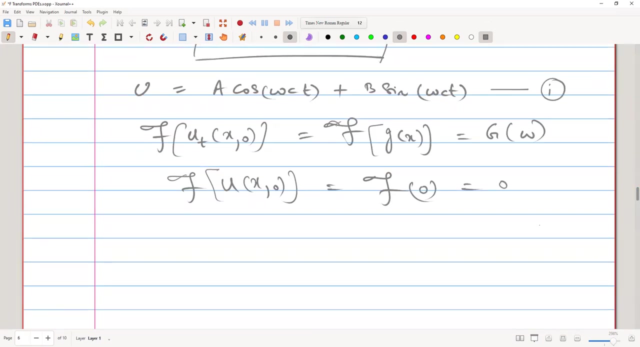 which is already zero. so we are going to get zero again. now we can apply these two uh uh conditions to this equation. let's call it, uh, this solution as one now put in these values here. so uh you be, first of all you need to calculate UT, or we can apply the first condition. so first condition: 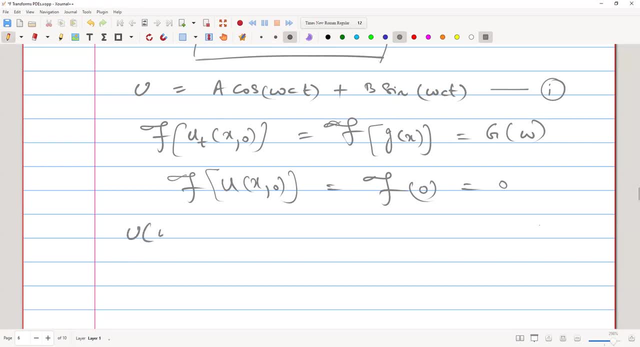 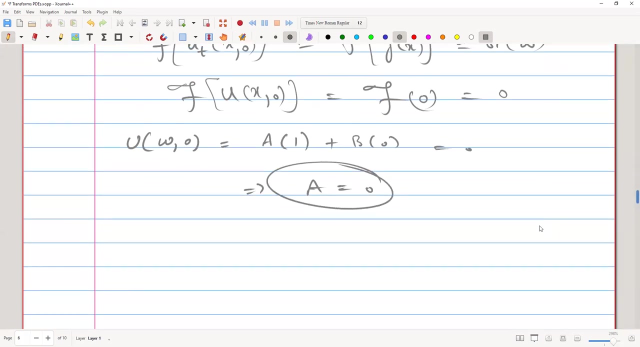 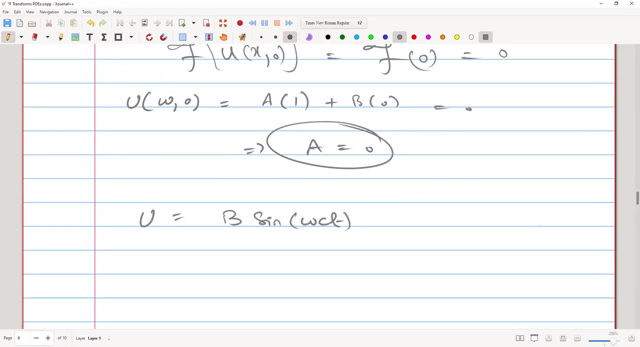 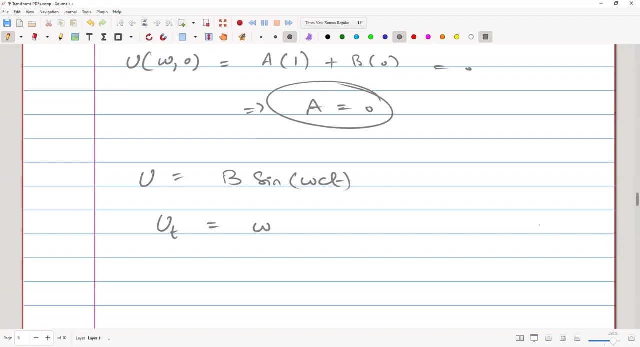 we can apply here, that is U of uh, Omega, comma, zero. it will be a times one plus B times zero, that is equals to zero, which implies that it's a equals zero. so now the equation becomes: u equals B, sine Omega C, T and simply uh. we can uh take the partial with respect to T for this equation, we will get Omega C. 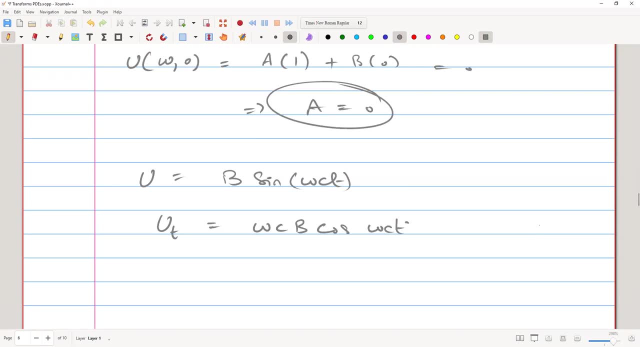 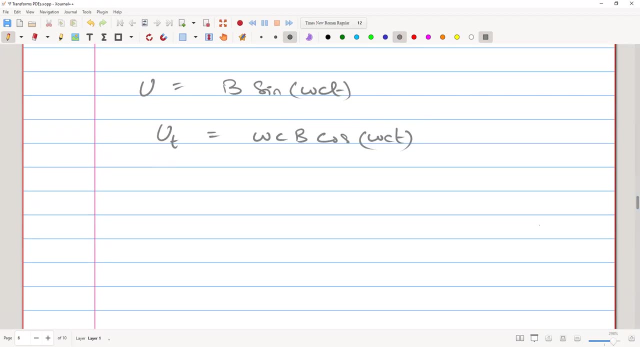 B cosine Omega C T and plug in the condition that is the initial condition to find this B. so U T of Omega comma zero is nothing, but it's G of Omega equals Omega C, B cosine zero. so this implies B equals G of Omega and one over Omega C here on the left. so this is the uh constant of the equation, what we get from. 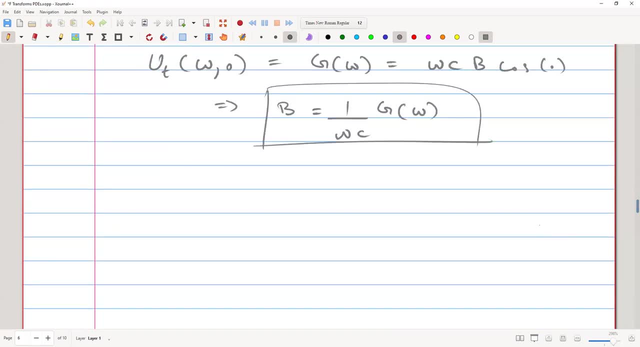 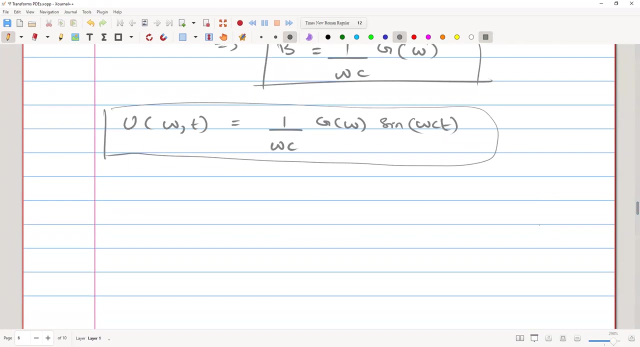 the condition, and then we can simply write: U of Omega comma T is equals to one over Omega C G, of Omega times sine Omega C T. so this is the solution of the equation in terms of Omega T, but we need the solution in terms of X comma T, right. 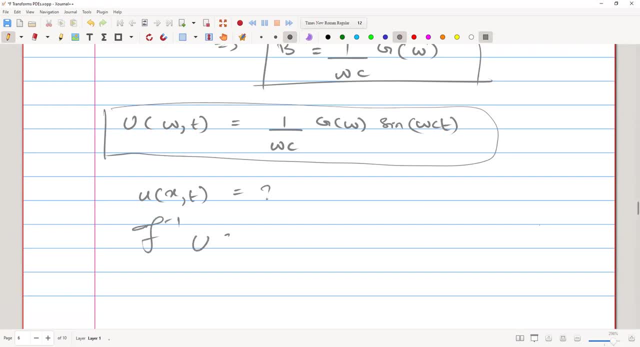 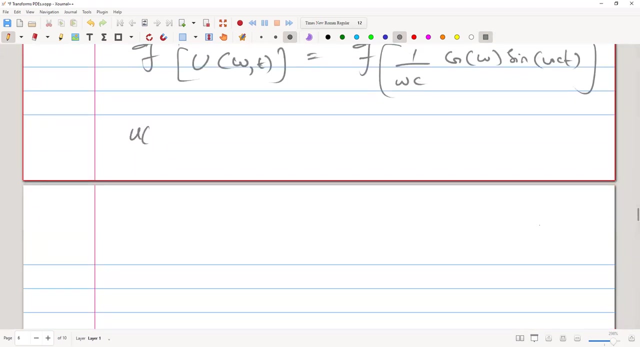 so, applying the inverse transformation to the equation, here we can write: inverse transforms, one over Omega C, G of Omega sine Omega C, T. so here we will have U of X comma T. now by applying the inverse transformation, and on the right side we can simply write Fourier inverse, and uh oh, it's one over Omega C. 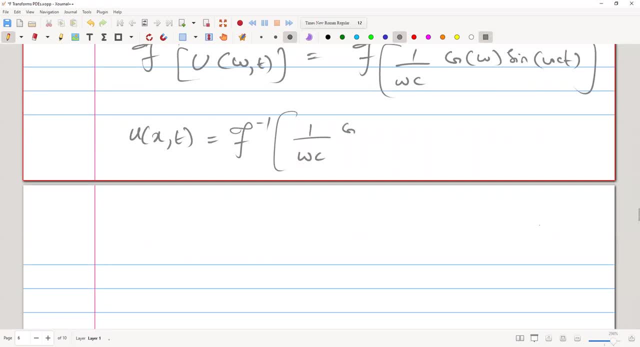 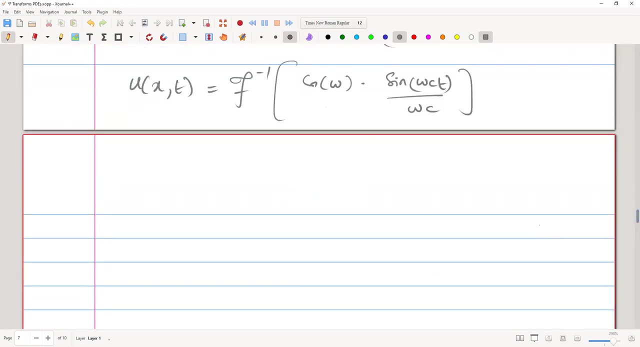 so one over Omega C G of Omega times, now for sine Omega C T. we can see here that this is okay. we should write in this manner so it will be easier to understand that this G Omega times sine Omega C T over Omega C. all right, so now what we can do here is we can simply: 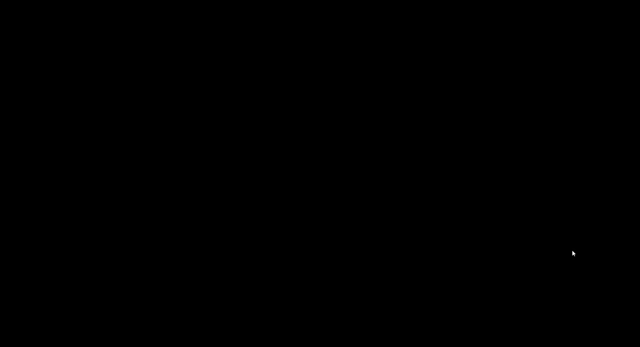 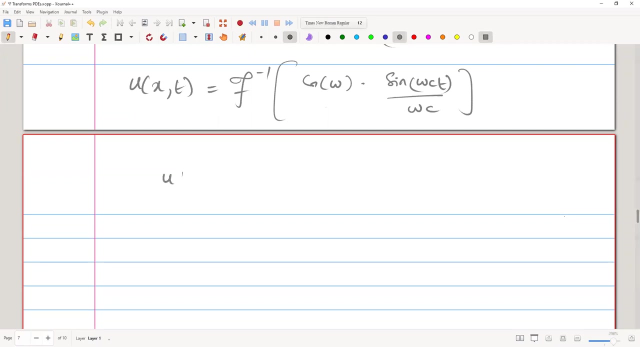 uh, now there is a result that we have already as, uh, we can do one thing here, and I will tell you how this will work. so this is G of Omega, and if I multiply two sine, sorry, if I multiply this sine Omega, C, T with two and again divide it with two, 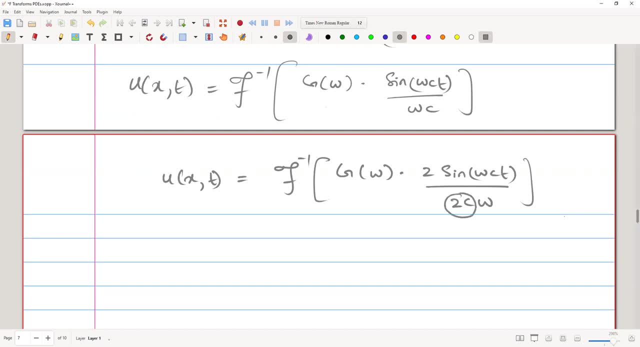 to balance the equation and then take this 2c outside and then i will show you what will happen. because this is the constant, so we can take it outside of the transformation and then we can apply the convolution theorem to this problem. so we can apply convolution. 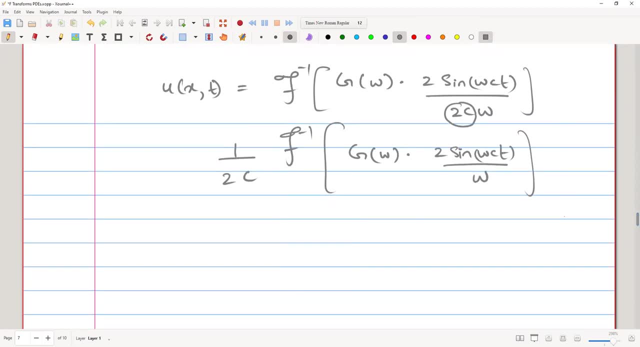 now we can apply convolution for this uh function inside and this will be 1 over 2c. and let me write here: a result from fourier transformation is that fourier inverse transform of this function two sine omega, c, t or omega. this is simply one. 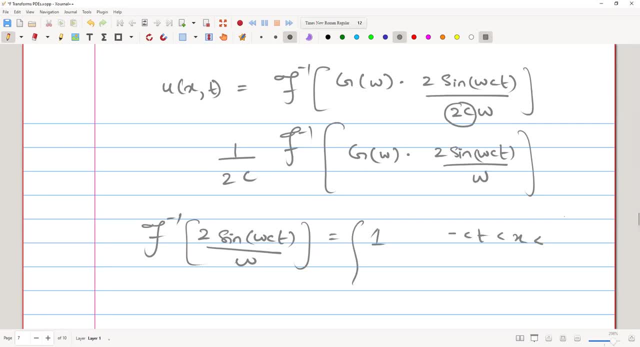 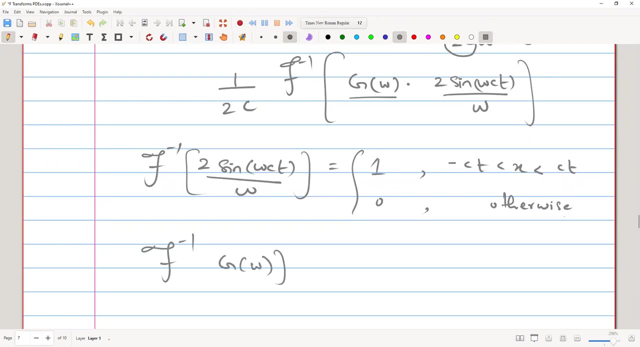 whenever x is between negative c t and positive c t and it's zero, otherwise right. so this is a result from fourier transformation, uh computations. so we know that the result of inverse of this transformation is this thing and inverse of this transformation, that is g of omega, this will be: 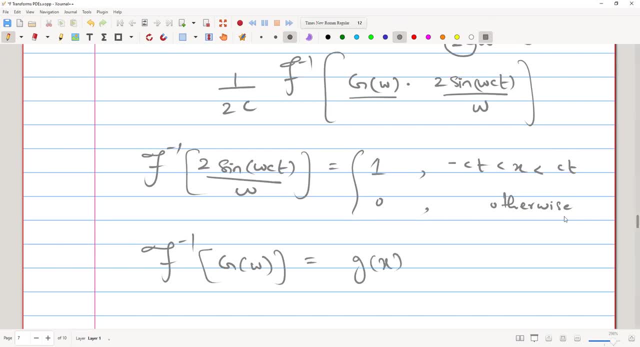 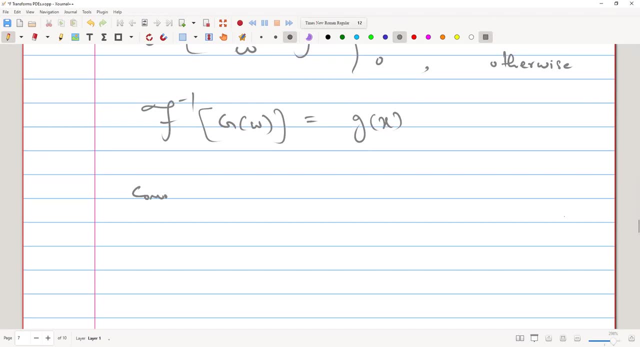 simply g of x again, so we can convolve these two things. so by using the convolution, convolution, so we can write this in a manner that u of x, comma t equals 1 over 2 c times g of x. convolution, f, inverse of whatever function we have to sign. 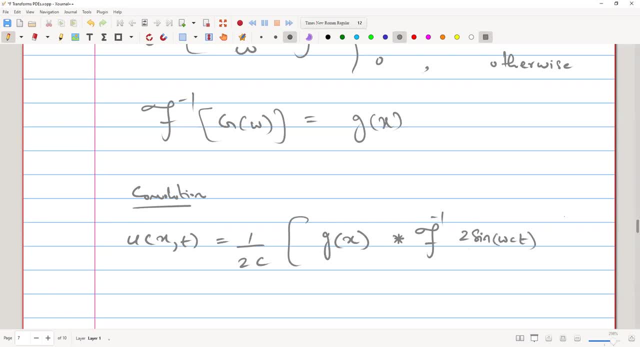 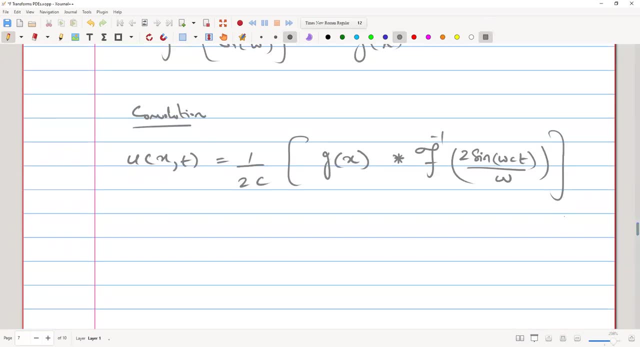 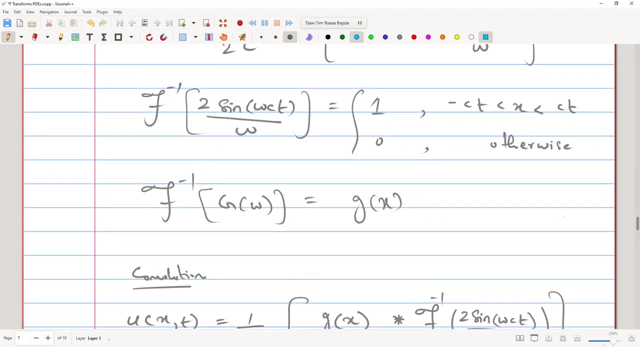 uh, omega, c, t over omega. so instead of the function i have written here, i write here this thing: right, so this, this is also inverse. we know that this is inverse of g, omega, and this is also inverse. we have a function here, this function, but it's a piecewise function. that's why i write in this manner, here to 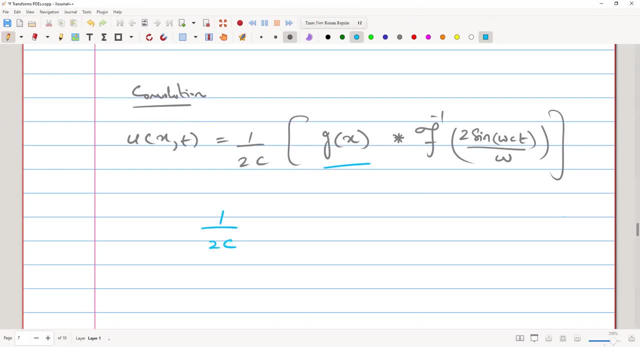 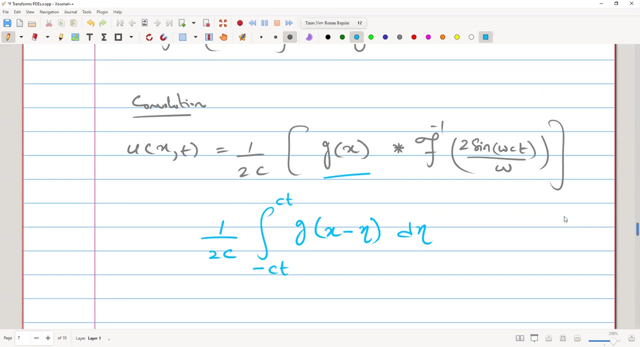 make it easier now. so i can write 1 over 2, c times the integral from negative c, t to c, t, g, of x minus eta, d, eta. so this is simply convolution and how i write this. uh, you just need to give some concentration here, right? we know that the function is, uh, the value. 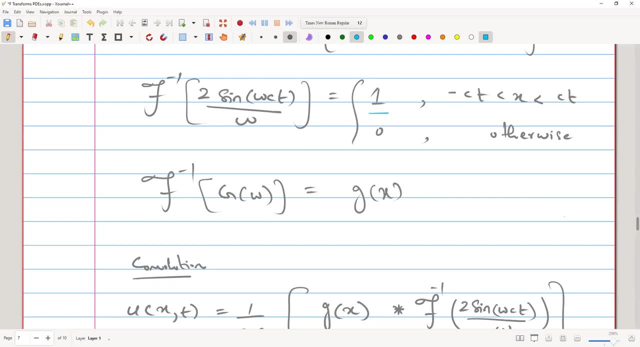 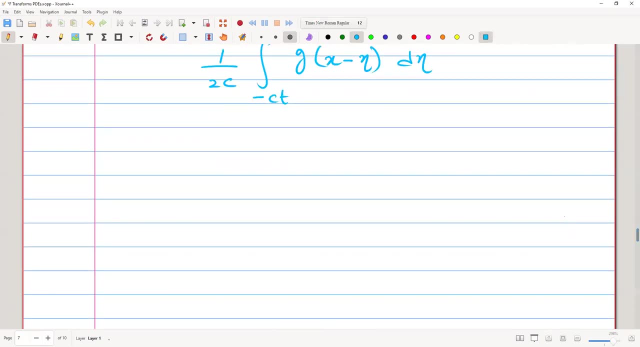 of the function inverse is one when it's between negative ct and ct and it's zero when it's otherwise right. so for the convolution, what we need to do is, if we have function f of x and we are convoluting it with g of x, uh f, from negative infinity to infinity, for instance d of x. so 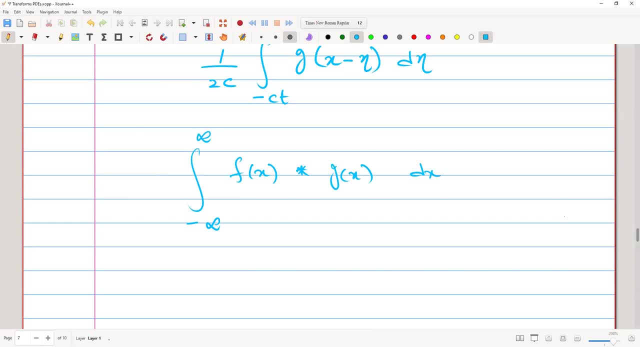 we write in this manner that it's: uh, we can write this convolution, uh, sorry, not, not like this the convolution. it will be like this: if we convolute f of x, convolution g of x, then we can write f of x here. we can see that g of x is g of x here. but for this f of x, f of x, we have one when it's: 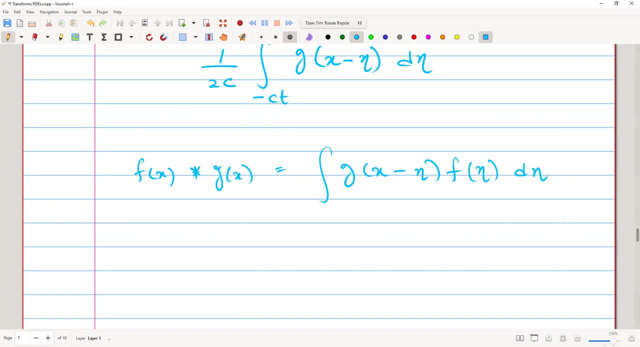 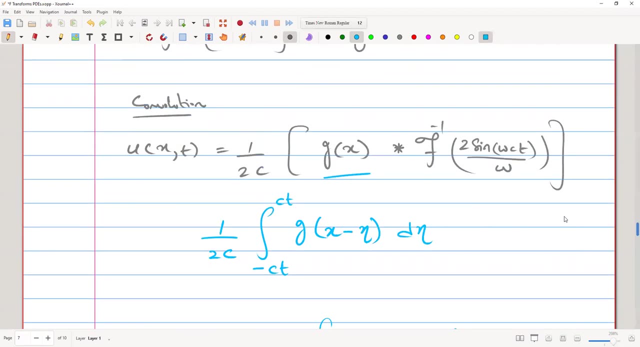 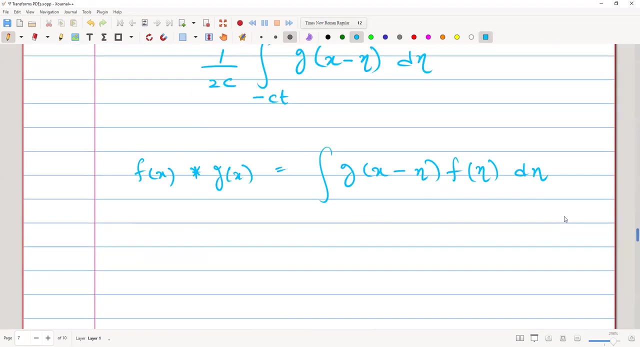 negative ct to ct. so, uh, we can write that as well, and we can write this as a integral. uh, we can write this as the integral uh, f of x, or we can simply say it as: that's why, when we convolute this one, this function here g of x or times like this, i can: 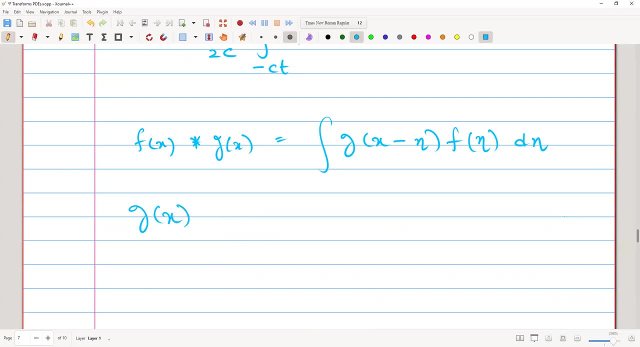 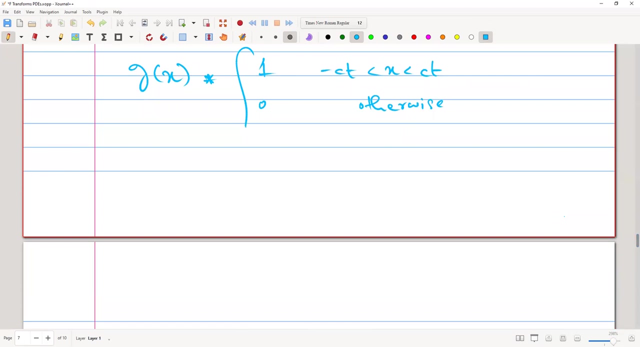 write it like this: it's g of x convolution the function, which is one when between negative ct and ct and it's zero otherwise. so i am convoluting this function in this manner. so now i can write it as from negative ct to ct and g of x minus eta, and instead of this that f of 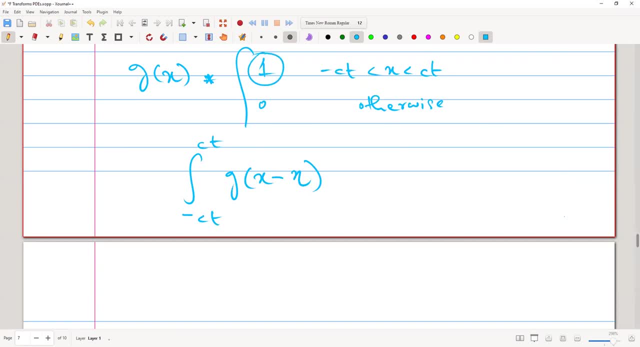 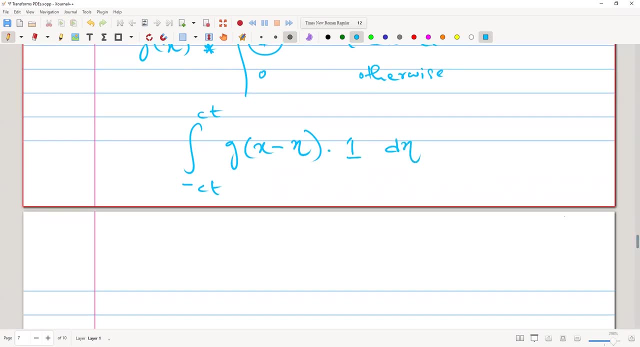 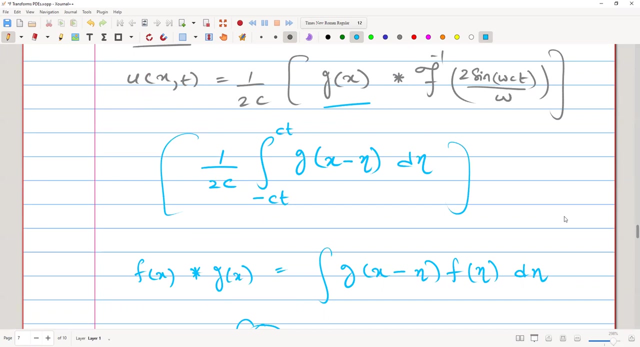 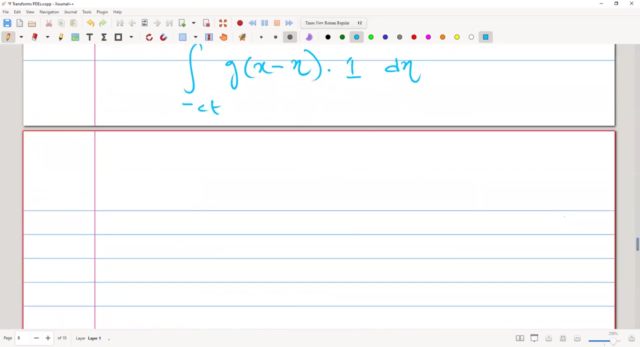 eta, sorry f of. yes, we have one here, so this will be simply one, and then the eta right. so now this: we can write here, as we saw earlier, that one over two c times this integral for this convolution. we can write by using the limits and then simply, what we are going to do is what we have is right now. 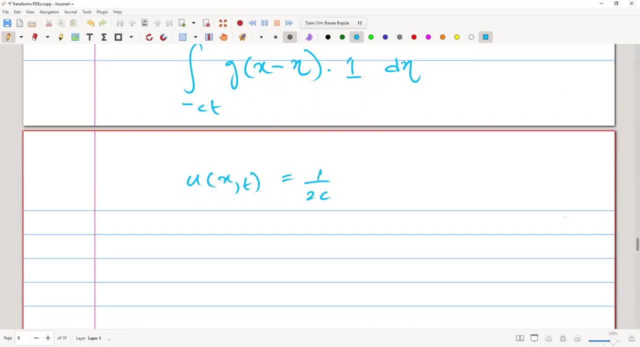 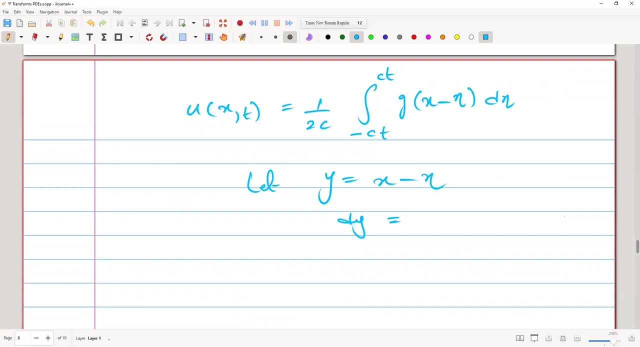 is: u of x, t equals one over two, c times the integral negative ct to ct. g of x minus eta times d eta, and so i'm going to suppose that let, for instance, y equals x minus eta, and so i know that it will be: dy equals uh dx, right, oh, sorry, not dx. uh dy equals d eta. 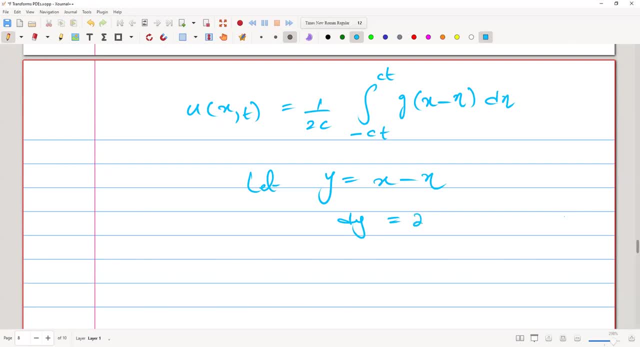 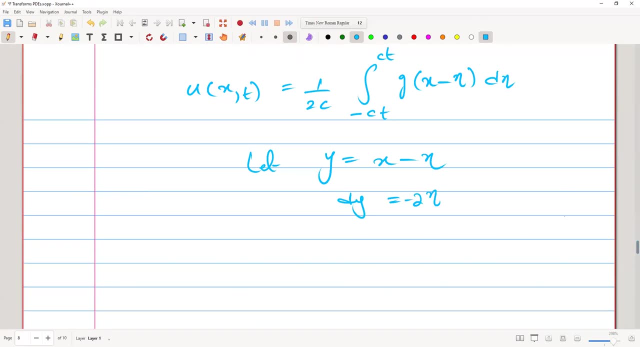 which we are differentiating with respect to eta. so it will be dy equal to d eta, with negative sign here. right, so it's negative sign. so the limits? now the limits. what about the limits? so limits are from negative cd to cd for eta. so i can plug in as x minus minus ct, which gives x plus ct. 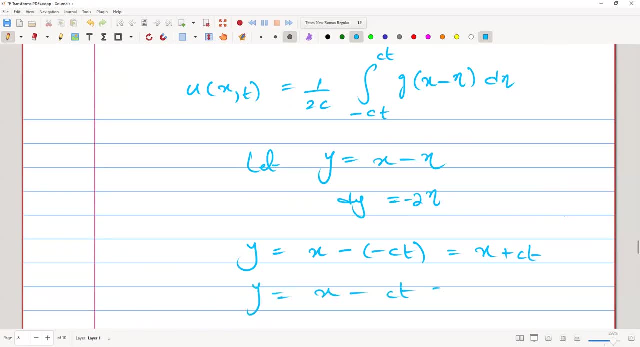 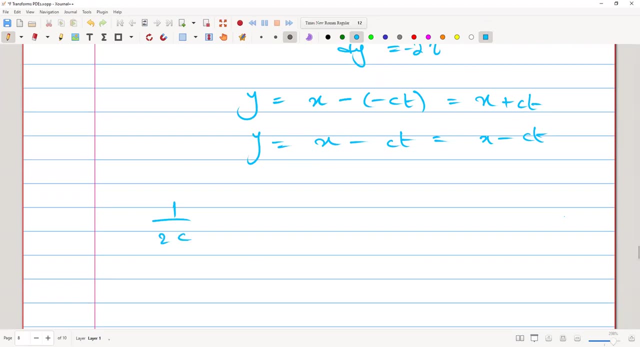 and then y equals x minus ct, which gives x minus ct. so now we can see the limits are from x minus cd to x plus ct, so it will be 1 over 2 c, x minus c t to x plus c t, and function is g of y. now 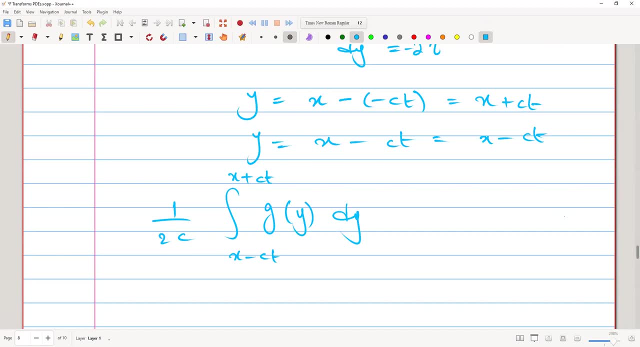 because we assume that uh, x minus eta equals y. so u of x comma t is equals to this integral. and here we go. we can saw that in the dlm birds, dlm burst, solution for the wave equation, we saw that uh, the solution for the initial displaced, initial velocity was given in this manner. so this also verifies that. 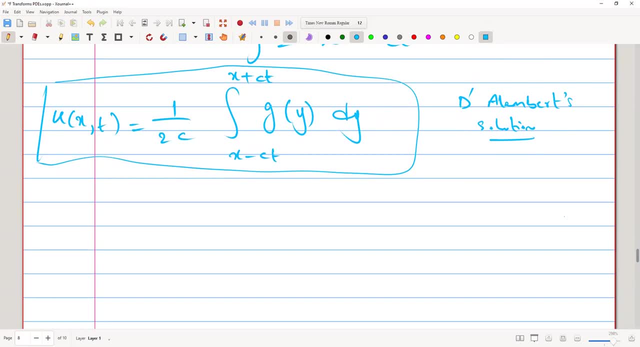 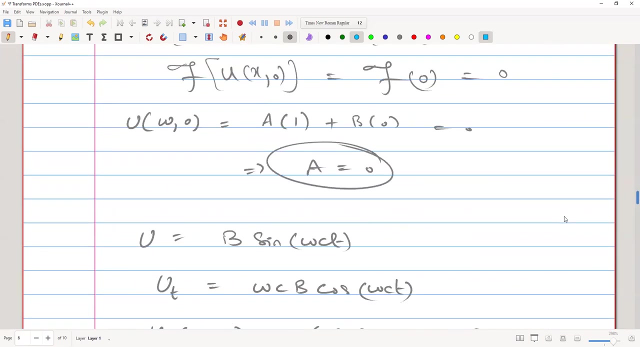 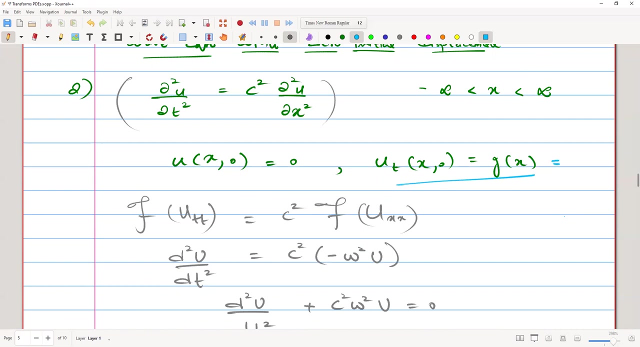 solution in general. this means that if you are given any function, any function of uh, y, let's say: if the function of uh, like i will show you here, like this, is uh. in the question we have uh, u or ut, x. comma 0 equals g of x, for instance. say that if it was x, let's say if it was x, for instance, 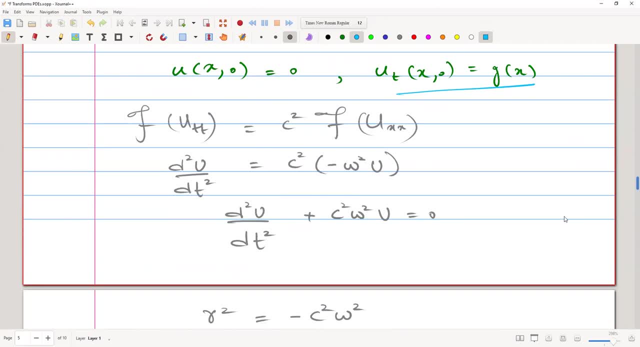 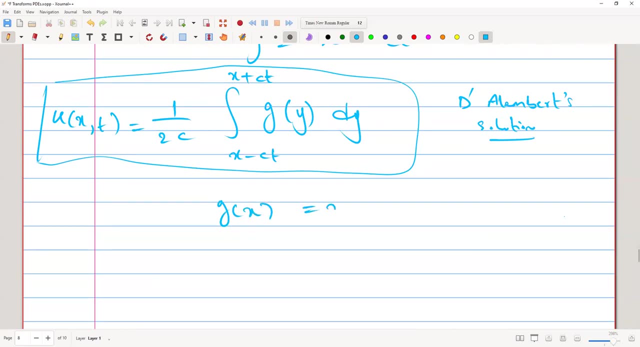 i will not write here, but, but we can see that if g of x was x, for instance, so what we need to do here? suppose that g of x was x, so g of y will be simply y, right, so now i can integrate this one over to c. 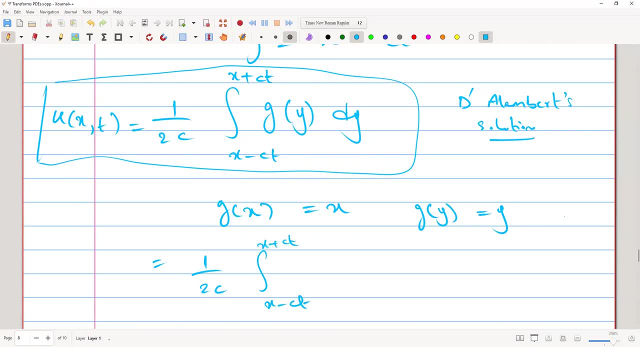 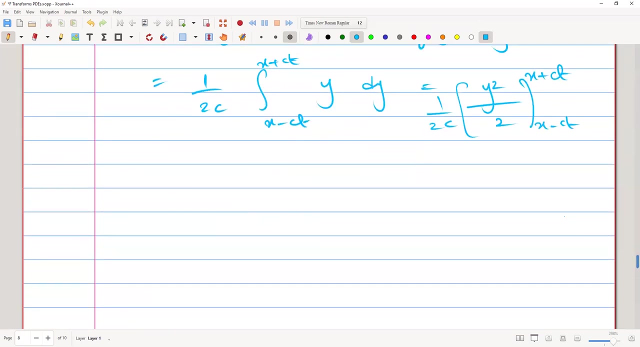 from x minus c t to x plus c t. g of y is y d y, which gives a solution: y squared over 2, 1 over 2 c limits from x minus c t to x plus c t, and we can see that this will be one over. 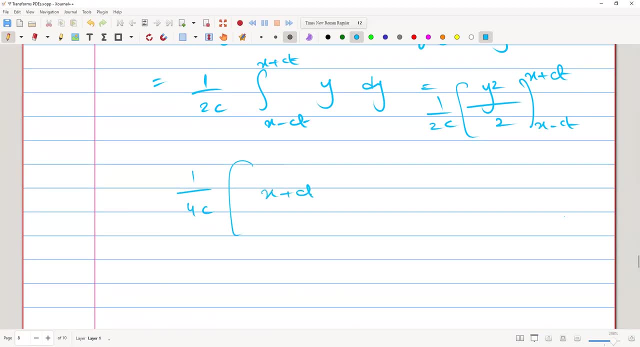 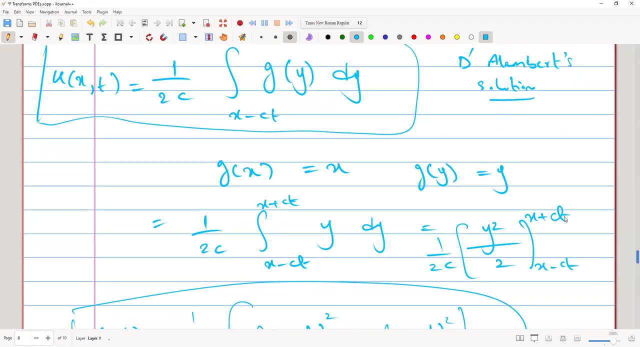 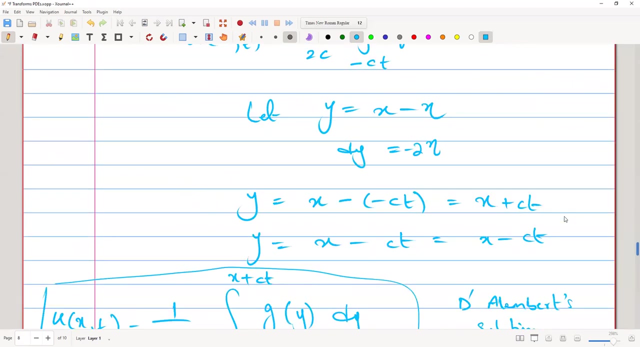 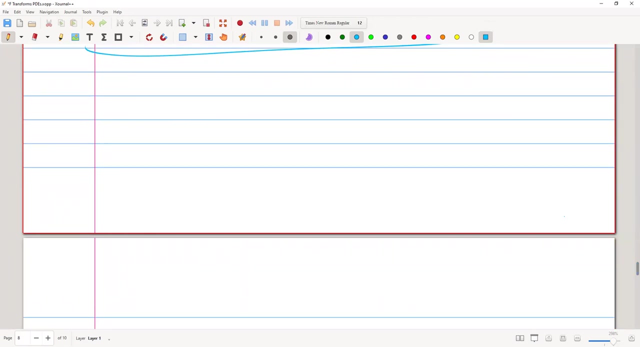 four c times x plus c t squared, minus x minus c t squared. and we can simplify further, but this will be the solution of the problem. so in general, we drive the solution for this wave equation when initial displacement is zero and initial velocity is some function of x, right, okay, so now. 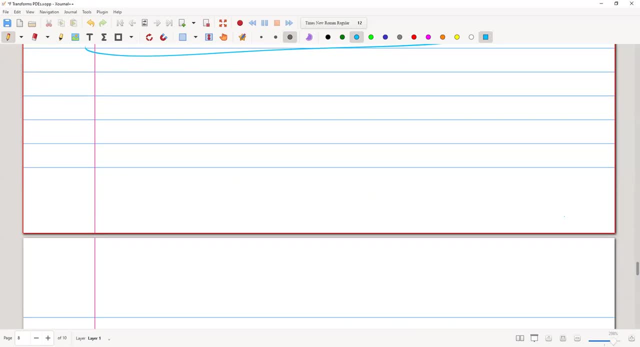 let's uh try one more problem. so it's uh heat equation. now we talk about the wave equation. now let's uh get to our heat equation. so it's dou u over our t equals c squared tau. squared u over dow x squared again the length of the rod. 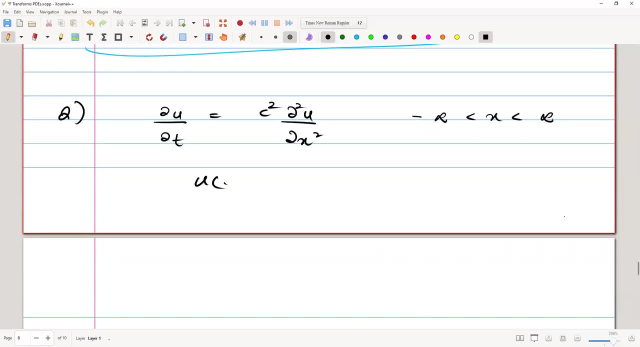 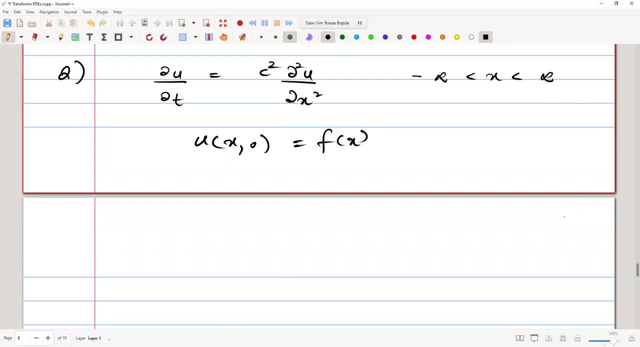 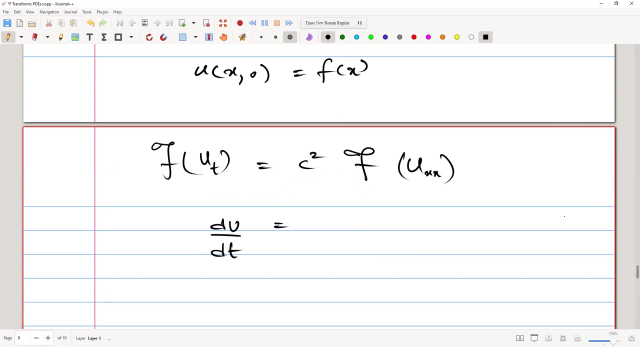 is from negative infinity to positive infinity. the initial condition is given as some function of x. so applying the transformation, we know that if we apply the transform on this equation here, we will simply get the result that we already discussed, and that will be: d? u over d. t equals c squared, negative omega squared. 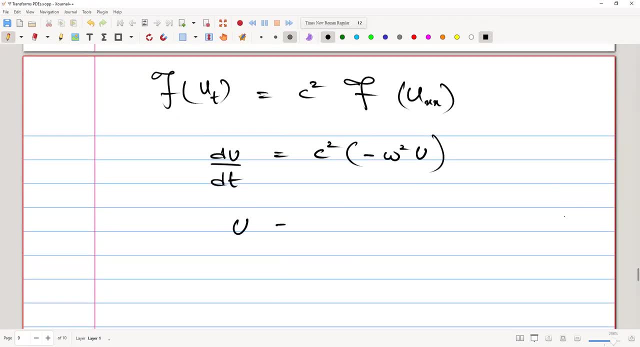 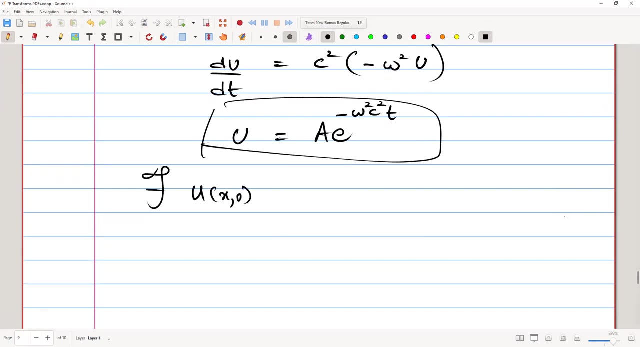 u. so when you solve this equation, we will get: u equals a, e raised to the power negative omega squared c, square t. now we need the initial condition. so apply the transformation to the initial condition. apply the transformation on f of x. we know we will get a function of omega. 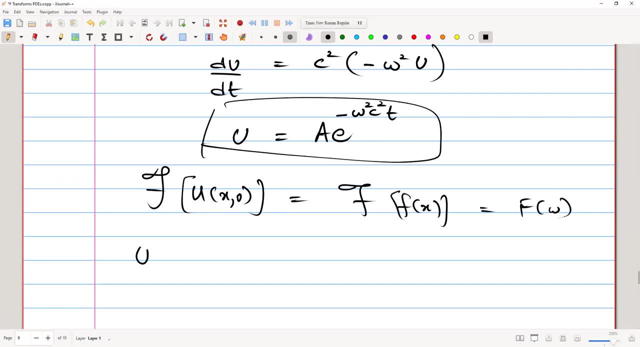 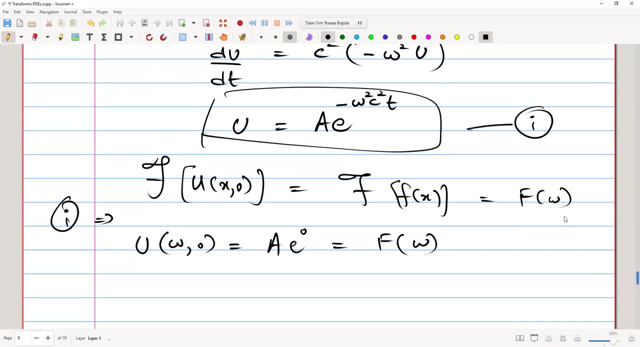 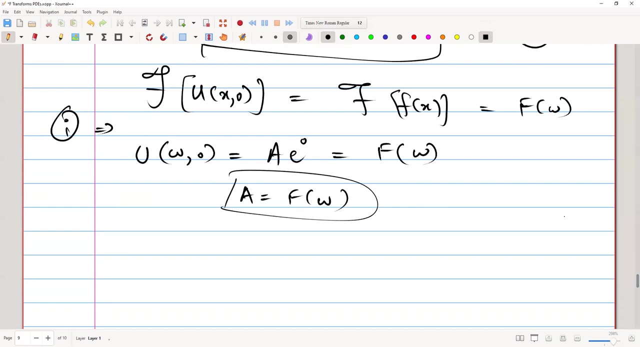 so we can write it as u of omega. comma. zero equals a. e to the power, zero is equals to f of omega. by using this equation, one right. so if i can write here, one implies: so a is equals to f of omega. a equals f of omega, so u equals f of omega. times here is to the power, negative omega squared c. 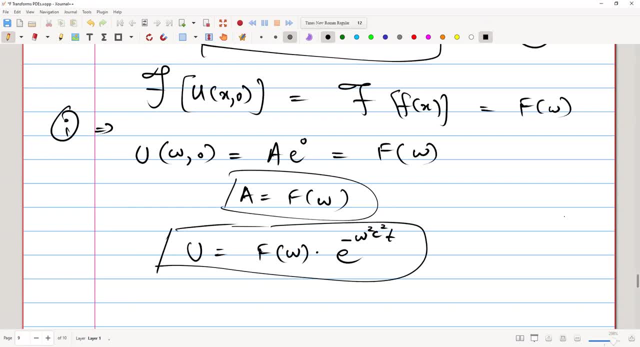 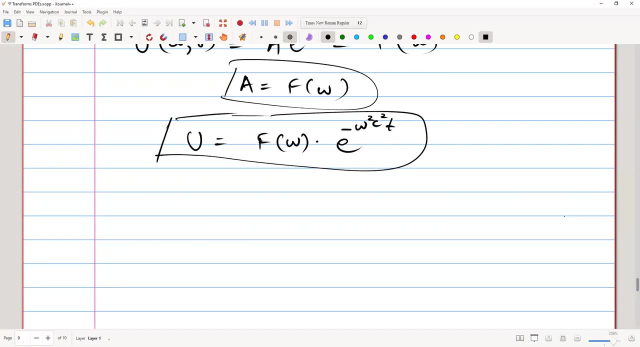 squared t. now again, we have a product function here, so we can use convolution to solve this problem. and or if we apply the inverse transformation on both sides, so it's a function of omega t, but we need a function of x t, so it will be negative omega squared c, squared t, so we can use convolution to solve this problem. 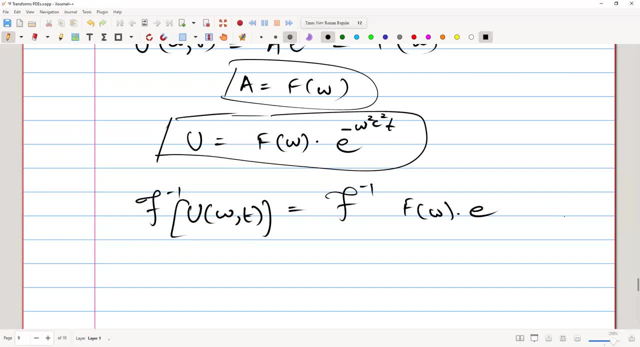 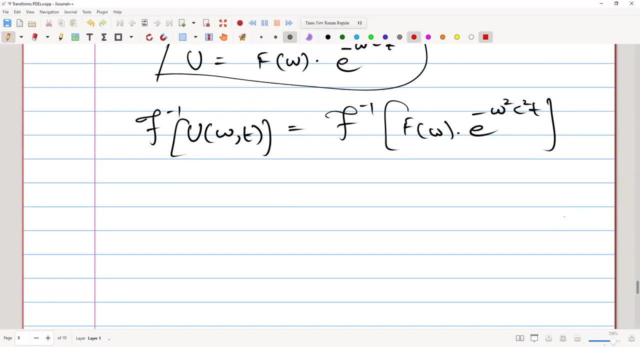 inverse f of omega times e, raised to the power negative omega, squared c, squared t, and again we will use our result from Fourier transformation. so i can write as now, that Fourier inverse of this f of omega will be nothing, but simply f of x, all right, and Fourier inverse of: 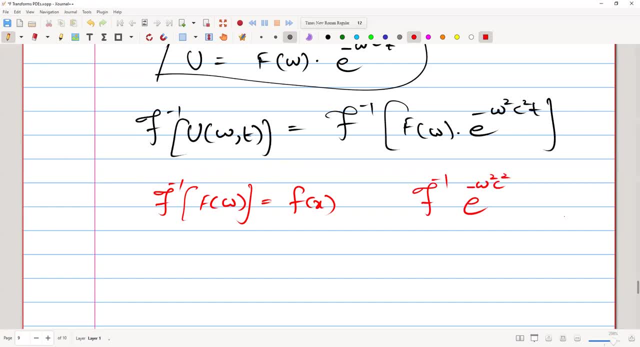 this function is also defined. so the Fourier inverse of this function, negative omega squared c squared t, or let's just keep it like this, and okay, we will progress in this manner first, then we will see the convolution first. we can just progress in the normal journal manner, so it will be simply 1 over 2. 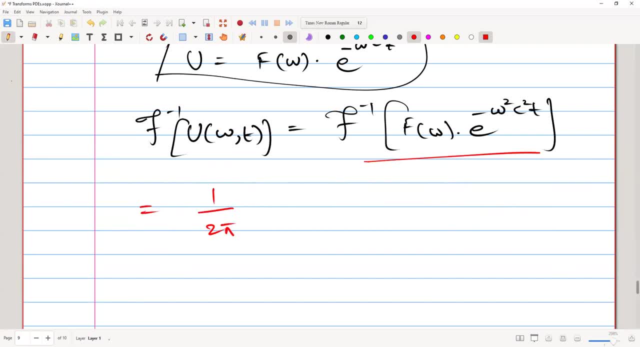 pi, this thing, this thing here, 1 or 2 pi from negative infinity to positive infinity, f of omega times, e to the power, negative omega, squared c, squared t times. e to the power, iota, omega, x, d, Omega. so this is u of x, alarm times, u, the power mater and the relationship between theta and gatherings. and now, if we write again also, so we can just progress in the normal journal manner, so it will be simply one over to pie, and now we'll今 e to the power undevi سے. we take f instead of here one over two by from negative infinity to positive infinity, f of omega times. a to the power, negative omega squared c, squared t times. e to the power omega xd, Vega. so this is, you have, a is grilled so that it's overall powered up. here once again, write and you'll get to theasil by the SLR formula. 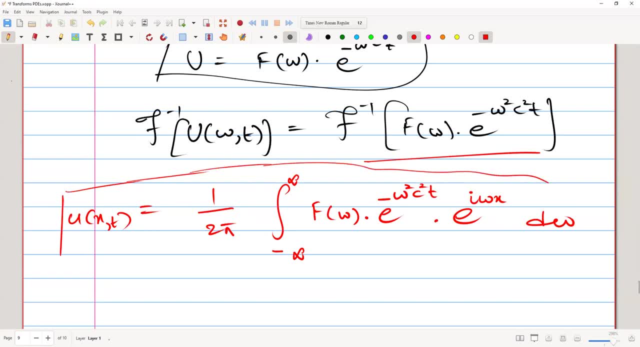 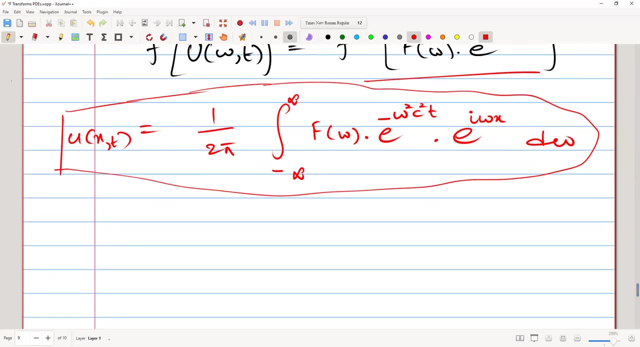 t. so we don't need to solve these integrals and for your transformations, it is enough to show in this manner, the integral manner, the solution. in this manner, it's fine, it's enough, right. and alternatively, if you want to use convolution, from here i will show you. 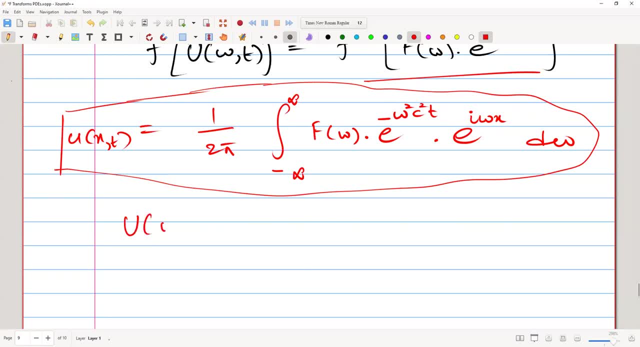 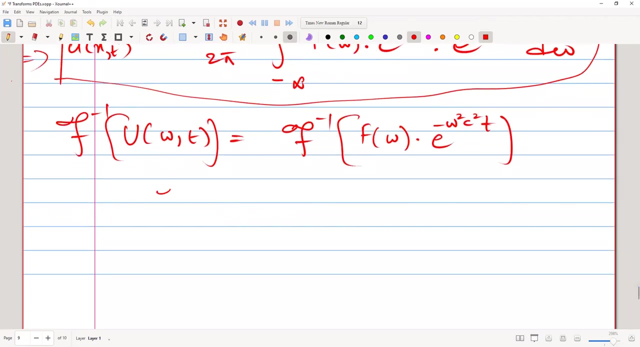 now up till here we have the solution. and one thing, one thing we have already seen, that is this one, and we can write the solution in this manner. and one more thing here is that if you write the solution by using convolution- so now we know that inverse of f of omega, it will be nothing but. 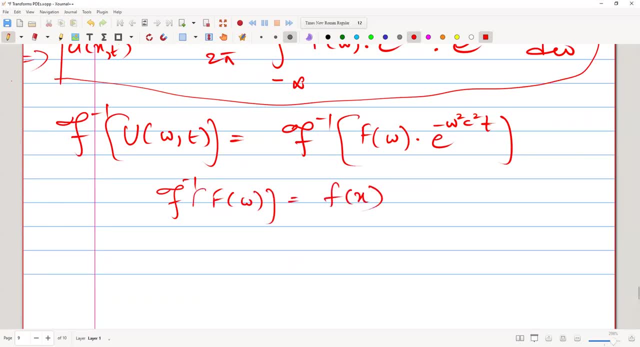 simply f of x, right, and the convolution, oh sorry, convolution, not convolution. inverse transformation of this function: negative omega c squared t, it will be. these are the results, right, uh, when we start solving fourier transformations. uh, in the next video lecture series, i will show you how these results come. 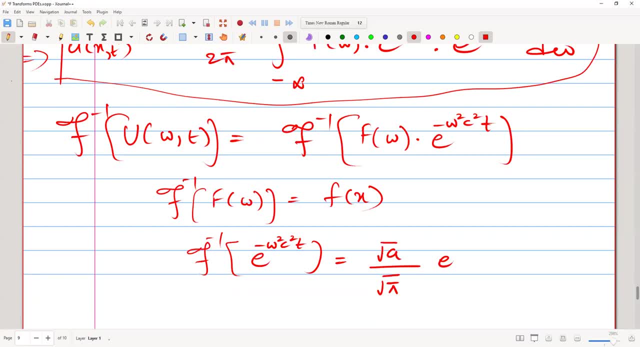 we can, how we get these results in this manner. right, so it will be simply okay, let me write a journal result first, journal results here, then i will show you so the inverse transform of a function, e to the power negative omega squared over 4 a is nothing but square root of. 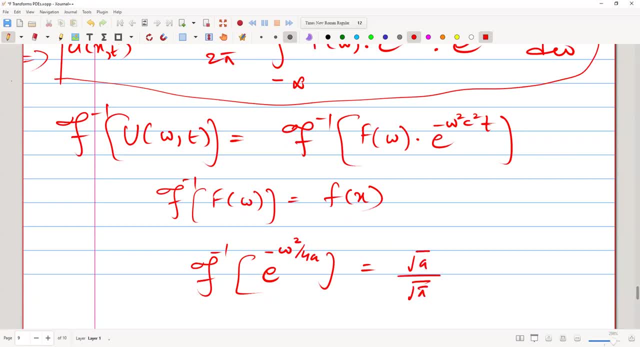 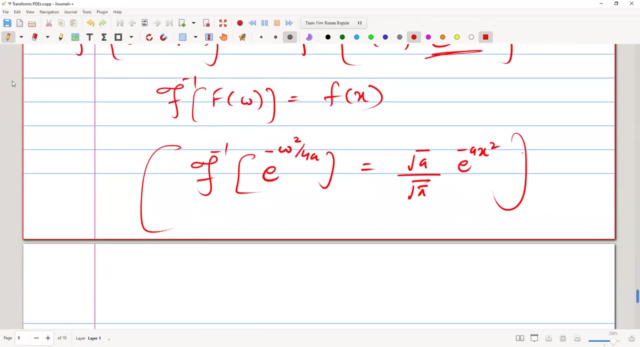 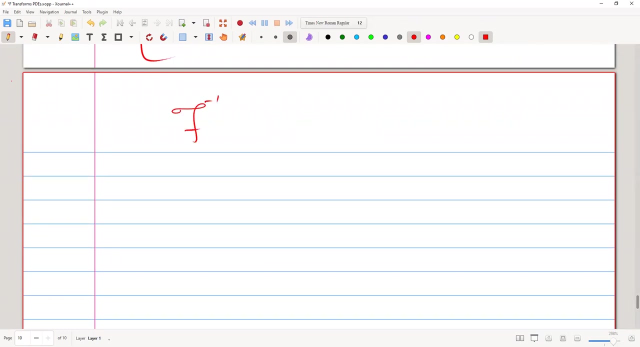 a over square root of pi times e to the power negative a square. so you can see this in the fourier transformation tables as well. this is provided. so now, by using this generalization, i will find the inverse transform of this function, so inverse transform of e to the power negative c squared. 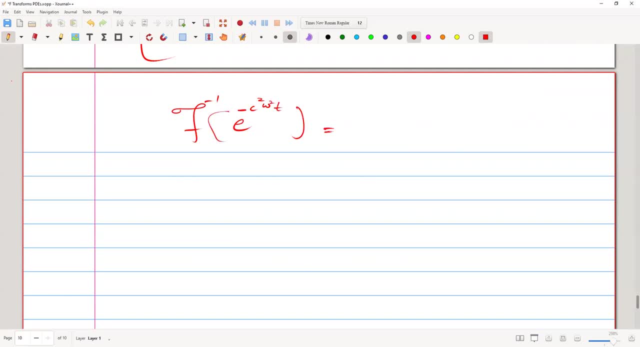 omega squared t, it will be equals to 1 over 2 c. square root of pi times t on t should be inside, not not outside. so it's pi t and exponential negative x is squared over 4 c square t. now we can conclude these two functions. so one of it is we get as f of x. 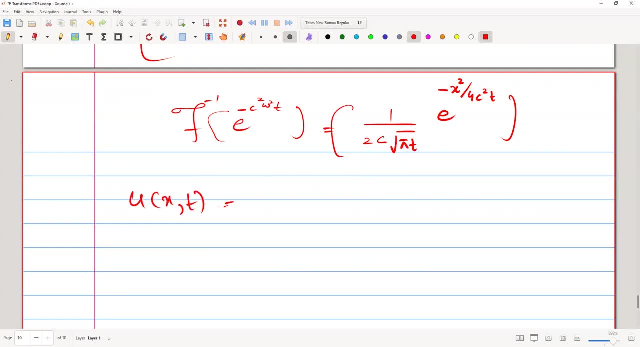 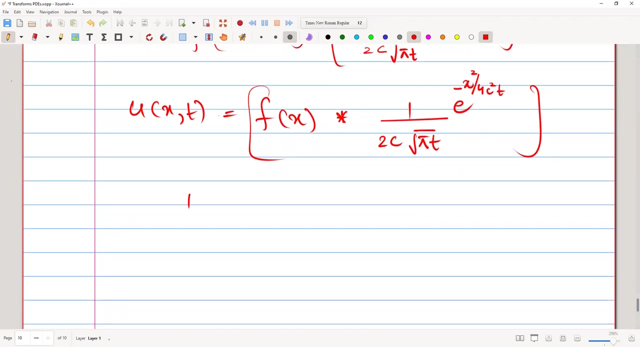 so we can write: u of x comma t equals f of x convolution. this function, that is 2 c square root of pi t, e to the power negative x squared over 4 c squared t into the power of 4 c square root of pi t in this operation. so for this function i will